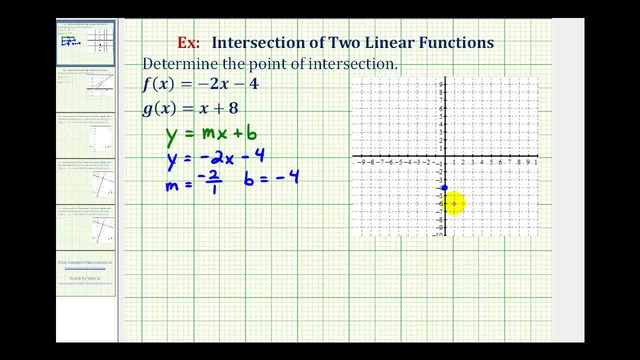 The slope is negative: 2 over 1.. So from here we go down 2, right 1, down 2, right 1.. And our line will pass through these three points. And for our second linear function, we can rewrite as: y equals x plus 8.. 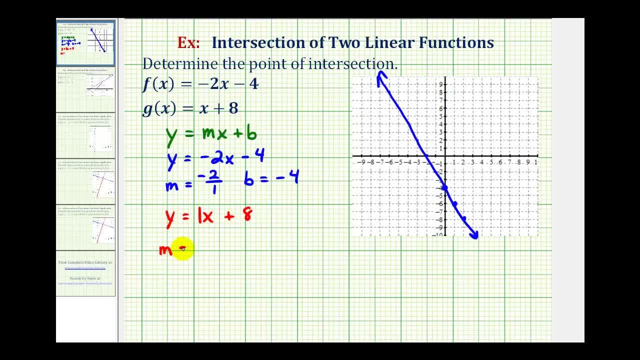 The coefficient of the x is 1.. Therefore, the slope of this line is 1, or 1 over 1. And the y-intercept is equal to positive 8.. Now we'll graph this line To determine the point of intersection. 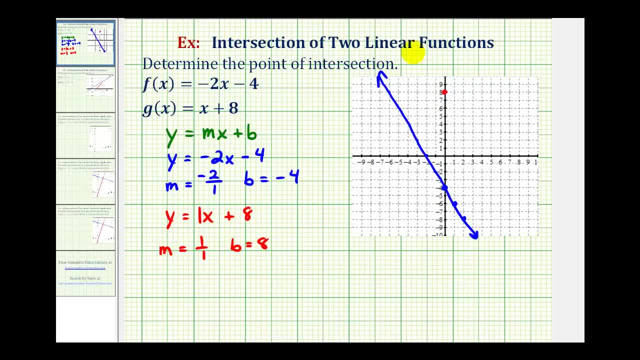 So here's our y-intercept: The slope is 1 over 1, so up 1,, right 1.. The second line will pass through these two points. Now that we've graphed the two lines, we can see the point of intersection would be this point here: 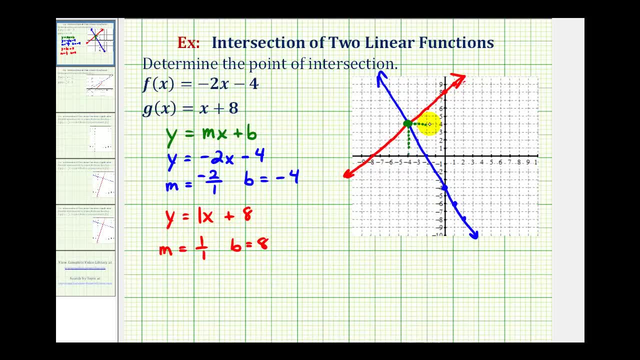 Where the x-coordinate is negative 4, and the y-coordinate is positive 4.. But graphing to determine points of intersection is often not the easiest method, because we have to graph very accurately And unless the point of intersection has integer coordinates, it's often difficult to determine the actual coordinates. 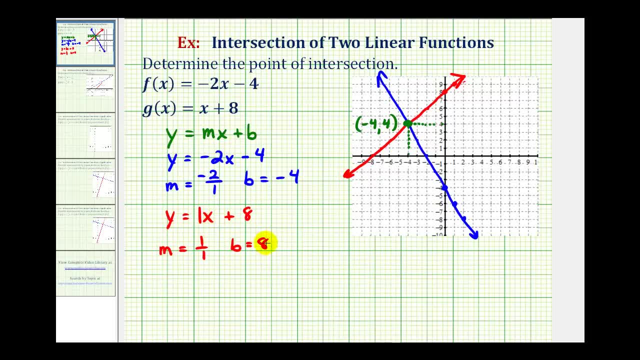 So let's also show how to solve this algebraically. To determine the point of intersection algebraically, we need to determine when these functions are equal to each other, Or when f of x is equal to g of x. Well, this is going to occur. 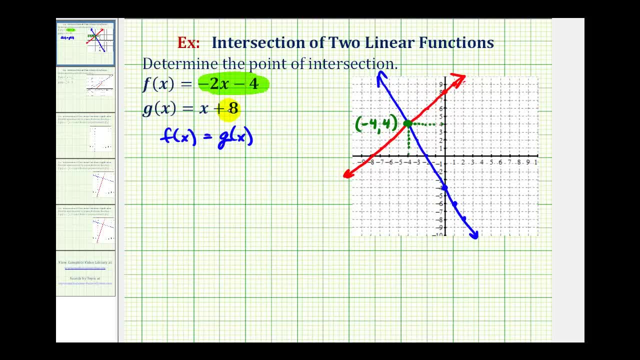 When negative 2x minus 4 is equal to x plus 8.. So let's go ahead and set up that equation and solve for x. So we'll go ahead and subtract x on both sides of the equation So we have negative 3x minus 4 equals. this would be 0, and then positive 8.. 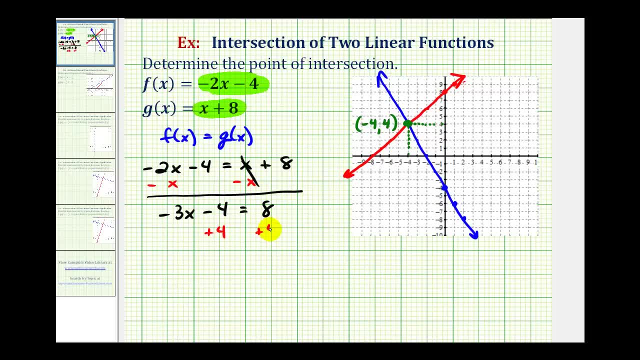 So add 4 to both sides, This would be 0. So we have negative 3x equals 12.. Divide both sides by negative 3. So we have x equals negative 4.. But remember we're looking for the point of intersection, so we need both the x-coordinate and y-coordinate.